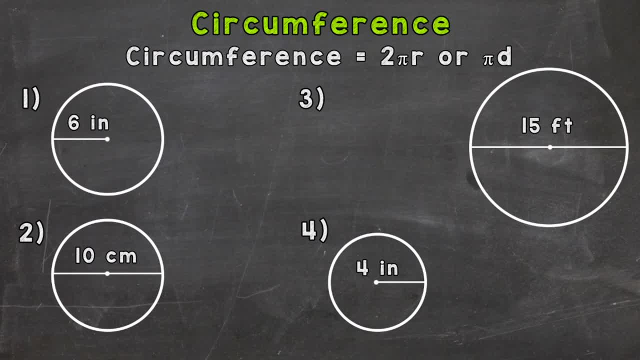 second here to the formulas, and we have this little symbol. we mentioned that that's the symbol for pi. Now, pi is the ratio of the circumference of a circle to its diameter. I'm just going to leave it at that. I'm not going to get into further detail about pi. There's great articles and 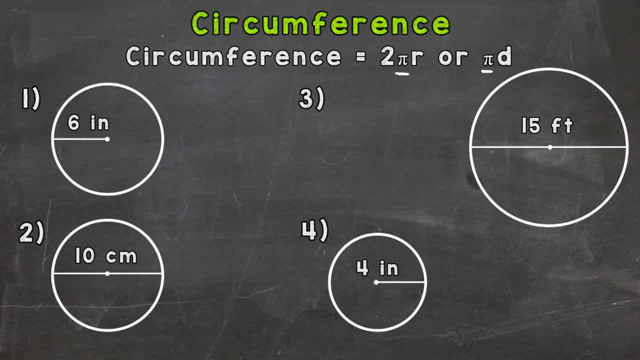 websites and YouTube videos that you can learn more about pi, but for now, we're just going to focus on calculating circumference. Now, pi is a very long decimal, so there should be a button on your calculator that you can use to calculate the circumference of a circle. Now, pi is a very long 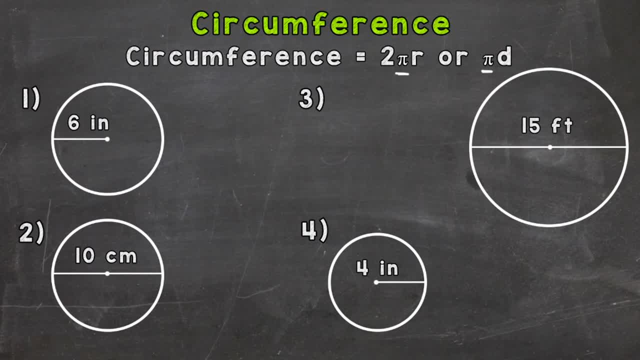 decimal, so there should be a button on your calculator that you can use to calculate circumference. as we're going through these problems, or it is common. since pi is a very long decimal, some people use the round rounded shortened version of 3 and 14 hundredths. Again, it's typical and common to 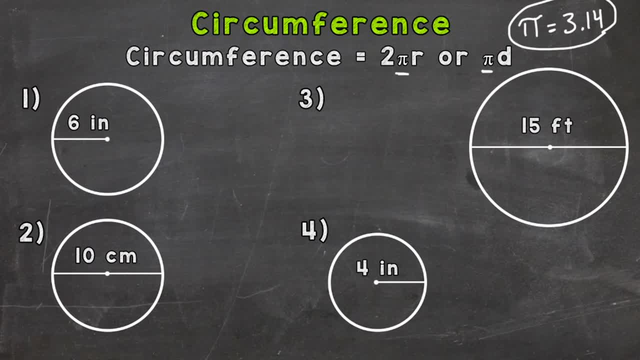 use that or use the button on a calculator. So let's get back to circumference here and, like I mentioned earlier, we have four circles or four problems on your screen That we are going to find the circumference for. so let's jump right in to number one. So for number, 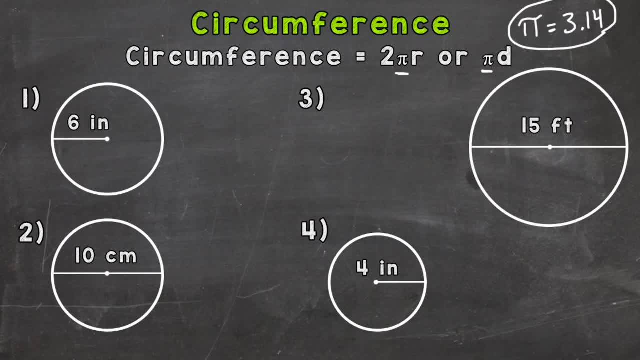 one. here we have a circle with a radius of six inches, and the first thing we want to do- it's always good habit- to write out your formula first. So we have circumference equals two times pi and we are given the radius, so I'm going to use the radius formula. Then let's plug in our radius. 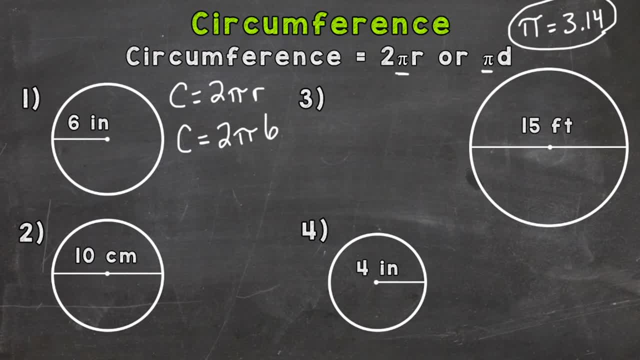 So two times pi, times our radius of six. Then we calculate, and once we punch it in to our calculator, we should get 37, and you're going to get a pretty long decimal there. so I rounded to the hundredths place, seventy hundredths, and our unit of measure is inches. Now one thing. 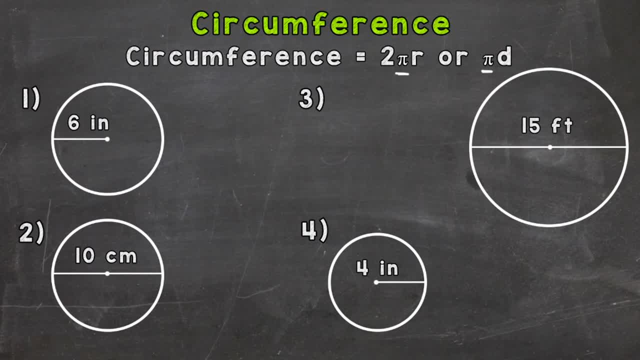 decimal, so there should be a button on your calculator that you can use to calculate circumference. as we're going through these problems, or it is common. since pi is a very long decimal, some people use the round rounded shortened version of 3 and 14 hundredths. Again, it's typical and common to 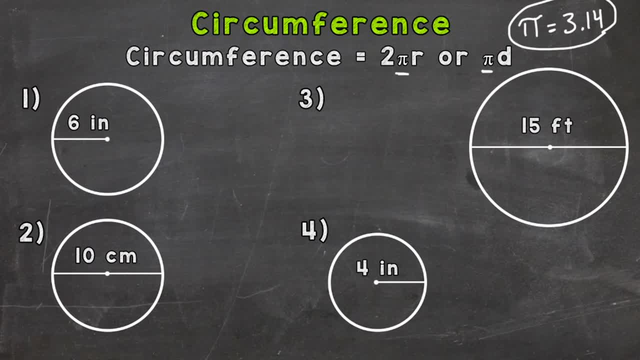 use that or use the button on a calculator. So let's get back to circumference here and, like I mentioned earlier, we have four circles or four problems on your screen That we are going to find the circumference for. so let's jump right in to number one. So for number, 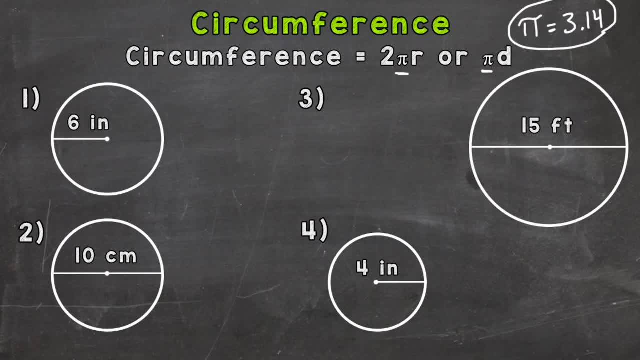 one. here we have a circle with a radius of six inches, and the first thing we want to do- it's always good habit- to write out your formula first. So we have circumference equals two times pi and we are given the radius, so I'm going to use the radius formula. Then let's plug in our radius. 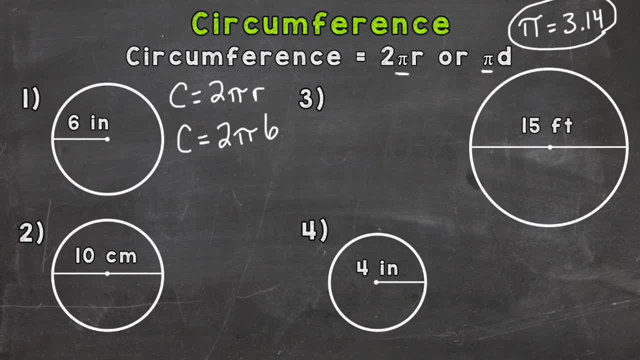 So two times pi, times our radius of six, Then we calculate and once we punch it in to our calculator we should get 37, and you're going to get a pretty long decimal there. so I rounded to the hundredths place seventy hundredths, and our unit of measure is inches. 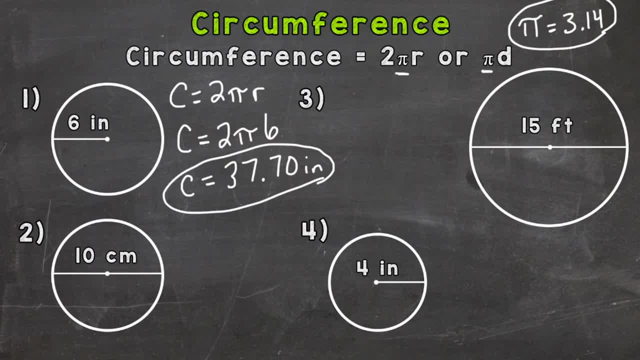 Now one thing I do want to mention. You can use either of these formulas, 2pi r or pi d, for any problem, Because if you're given a radius, you can find the diameter. you just double the radius, right. It's six inches halfway across this circle, so all the way across, the diameter would be 12 inches. 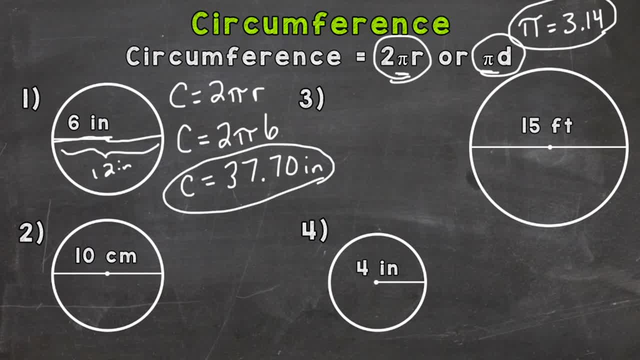 So you could do pi times 12 and it would give you that same answer. Or, given a diameter, you can have it. cut it in half and you would have the radius and you could use the 2 pi r. so both formulas are essentially the same thing, just depends if you use the radius or 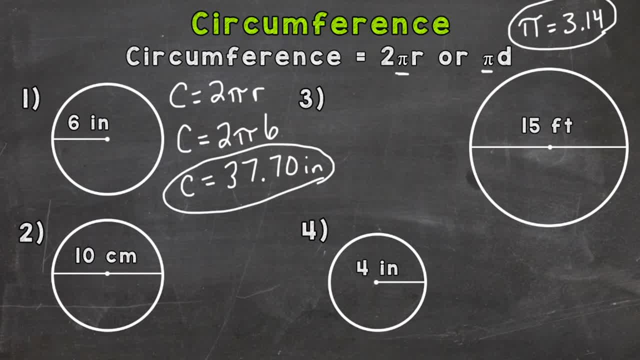 I do want to mention. you can use either of these formulas- 2, pi r or pi d- for any problem, because if you're given a radius, you can find the diameter. you just double the radius right. It's six inches halfway across this circle, so all the way across the diameter would be twelve inches, So you could. 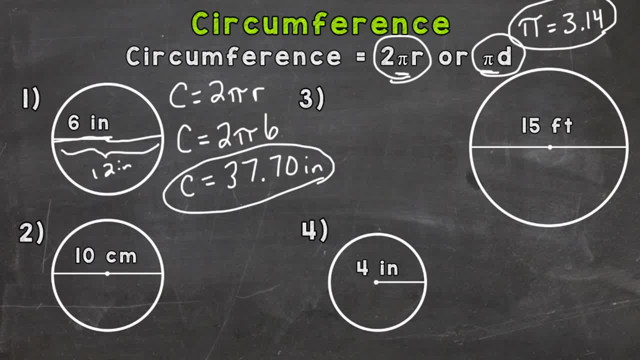 do pi times twelve and it would give you that same answer. Or if you're given a diameter, you can have it. cut it in half and you would have the radius and you could use the two pi r. So both formulas are essentially the same thing, just depends if you use the radius or diameter. 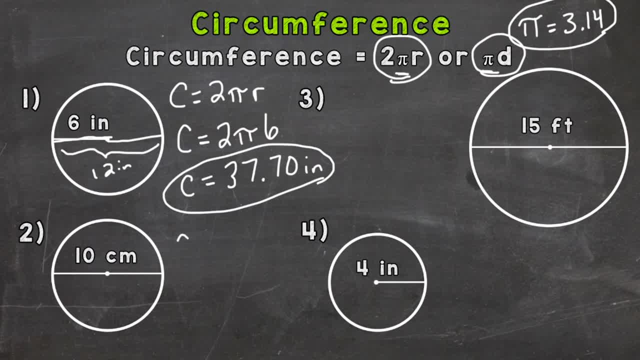 So let's go to number two. here, Circumference equals, they give us the diameter, so let's use pi times diameter. Next step, let's plug in: we have pi times the diameter of 10 centimeters. then we calculate and we get an answer of 31 and 46 hundredths. 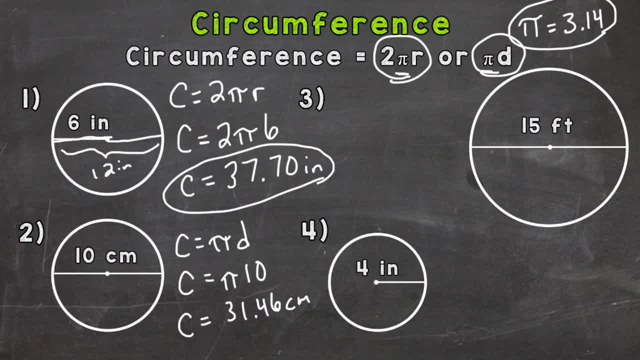 centimeters. again, this one gave a long decimal, so I rounded to the hundredths place. number three: we are given the diameter, so let's use: circumference equals pi D or pi times diameter. we'll plug in the diameter, so pi times 15, and then calculate and we get an answer of 47 and 12 hundredths, and this is feet. 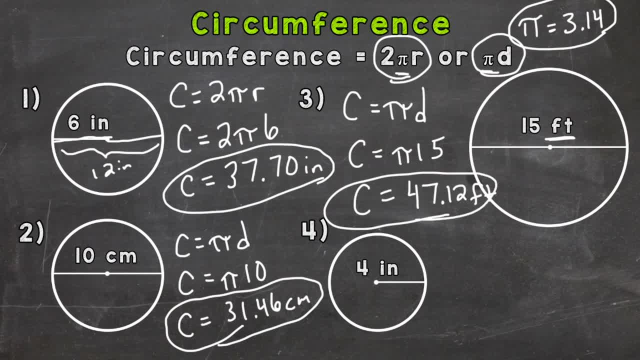 again, just to recap, circumference is the distance around the circle, so the perimeter. so if I were to trace, we're going to go around- I'm not drawing a perfect circle here, but go around that circle it's. the distance around would be 47 and 12 hundredths feet. number four, let's